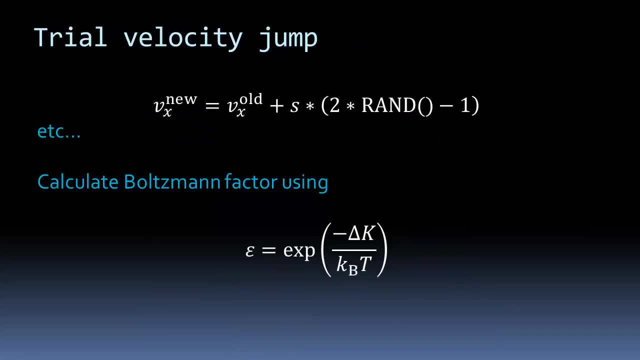 Now, to do this, we're going to have to step through and generate trial velocities, And the way we're going to do that is, for each component of our three dimensional gas, we're going to calculate the new value of the velocity from the old one by taking a random step of 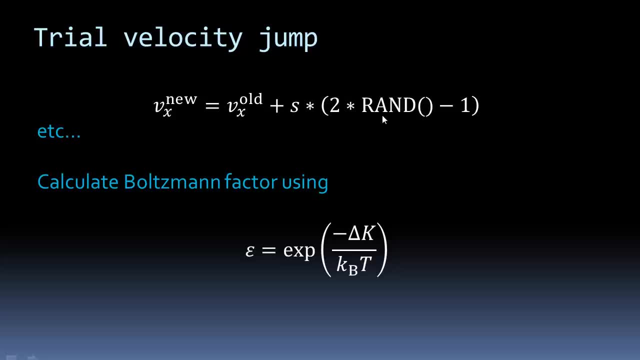 size minus s to plus s, which is how this thing works. You'll maybe remember that from the previous video. Then what we're going to do is calculate the Boltzmann factor, for the kinetic energy change is just minus of the kinetic energy divided by the thermal energy. We can then use the 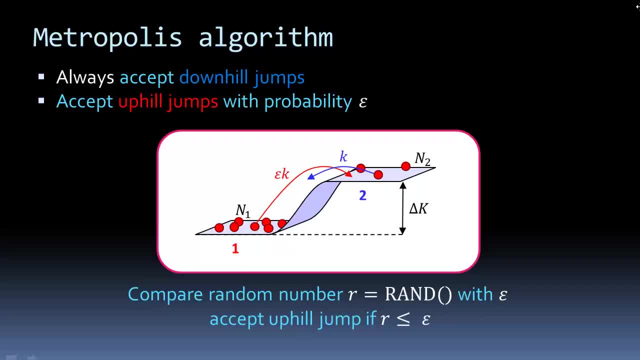 metropolis algorithm to decide whether the change in kinetic energy will occur. For downwards jumps it's always accepted, so those always occur. but if we're jumping uphill in energy, then those jumps have to occur with a fraction- epsilon- and the way we're going to do that is by comparing a random 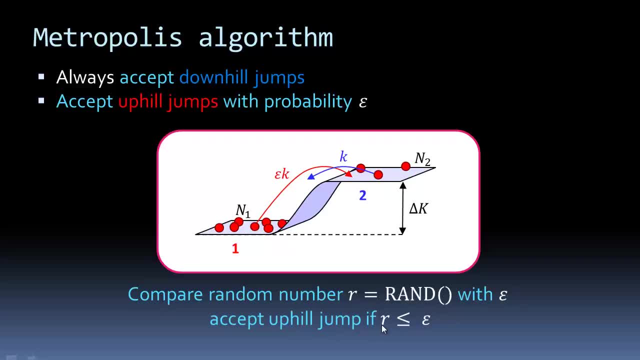 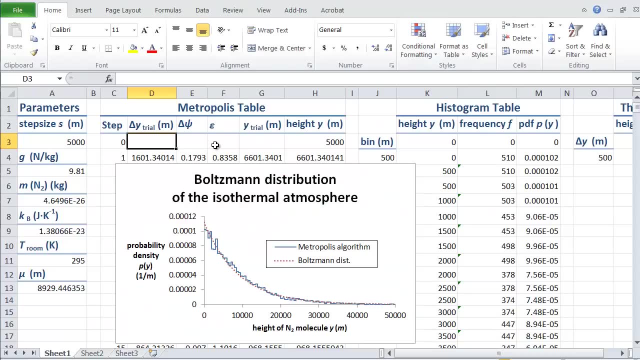 number r with epsilon, and if the random number is less than or equal to epsilon, then we'll accept the jump. otherwise, we'll stay at the same kinetic energy. Okay, so I'm going to start by showing you the spreadsheet that we generated at the end of the last video, where we generated the Boltzmann. 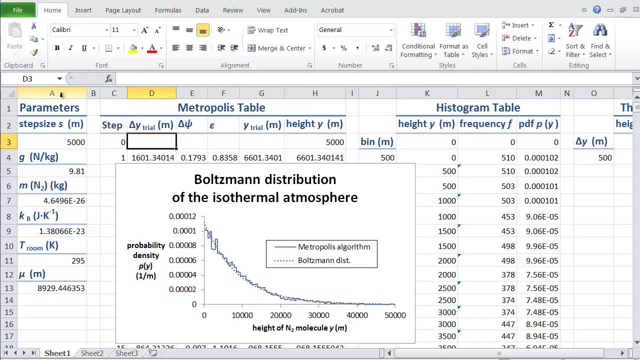 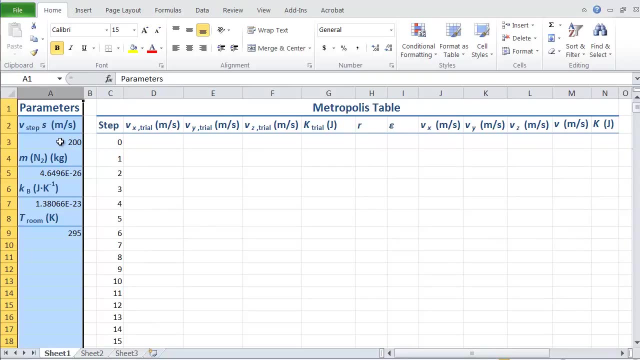 distribution for the isothermal atmosphere. Now what I'm going to do is I'm going to trim off all the stuff that we don't need and redo all the headings to match our new number. So we're going to start by doing the same simulation, and here it is. we have a parameters column which now has the step in velocity, which we're going to make: 200 meters per second. We've got the mass of the nitrogen molecules in the gas, a Boltzmann's constant and the temperature in kelvins. What I've also done is in the step column- here I'm just counting from zero down to 10,000 and in step zero I'm going to set up. I don't need anything for these first few things, but I do need an initial velocity for the step. So I'm going to set up a step column here and I'm going to count from zero down to 10,000 and in step zero I'm going to set up. I don't need anything for these first few things, but I do need an initial velocity for the step. 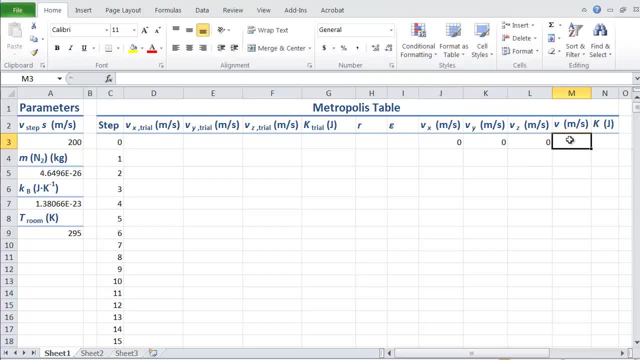 So I'm going to set up a step column here and I'm going to count from zero down to 10,000 and in step zero I'm going to set up. I don't need anything for these first few things, but I do need an initial velocity for the step. 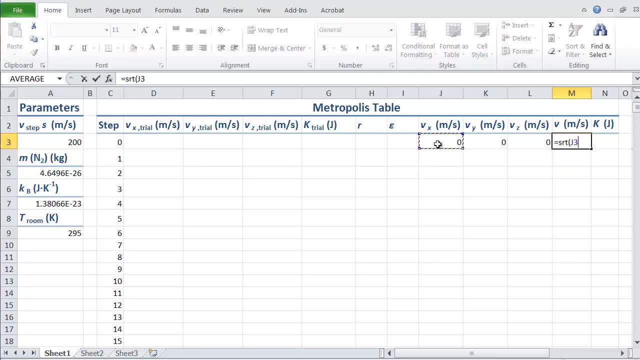 Then I need to calculate what that is by going. it's equal to the square root of x squared, which I can do by just multiplying it by itself, plus y squared, plus z squared, and then close, paren, And I have an error. it should be square root, so sqrt. there we go. 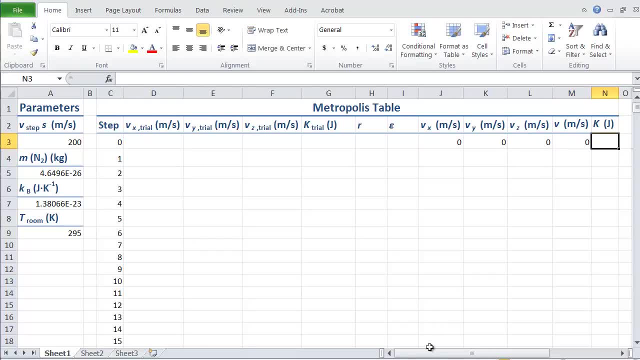 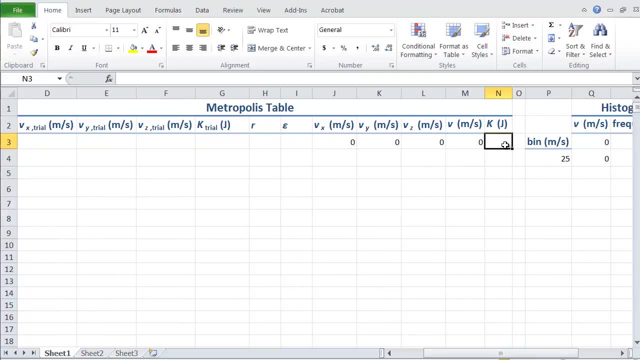 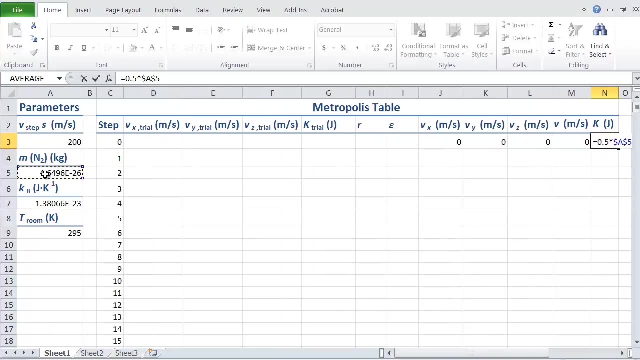 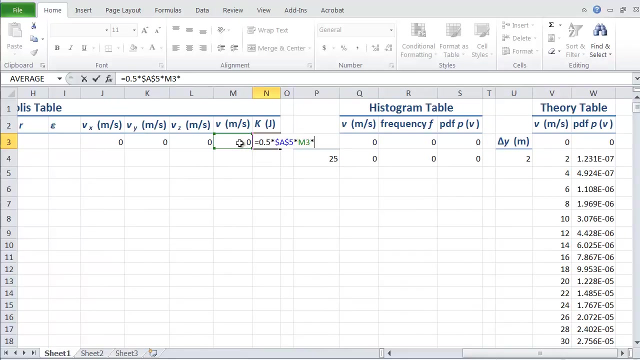 And then finally, finally, what I need to do here is calculate the kinetic energy, and that, of course, we can use our familiar formula from physics: 1, which is equals one half times m, which is way over here. hit f4 to get it all the time times v squared. so times v times v. Okay. so now let's do our first step. 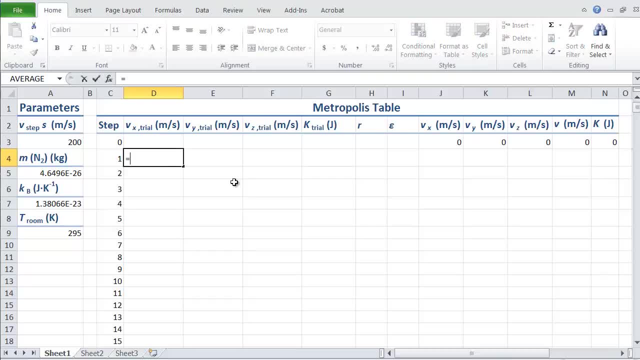 in the metropolis algorithm. so what we need to do is we're going to make the new trial velocity equal to the old one plus the step size, and we have to hit f4 times our random thing, which is going to be 2 times rand minus 1- close paren, close paren, and so that gives us a random. 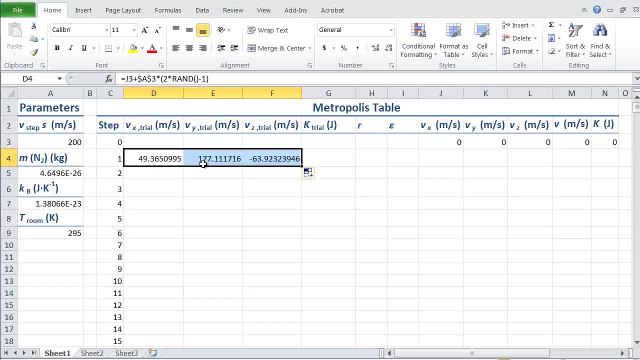 number, and we want to do the same thing for y and z. So we get three different random values of the, the trial velocity components. so we need to calculate the kinetic energy, which is, of course, is equal to one half times m hit f4 times all of the velocity components squared, so vx. 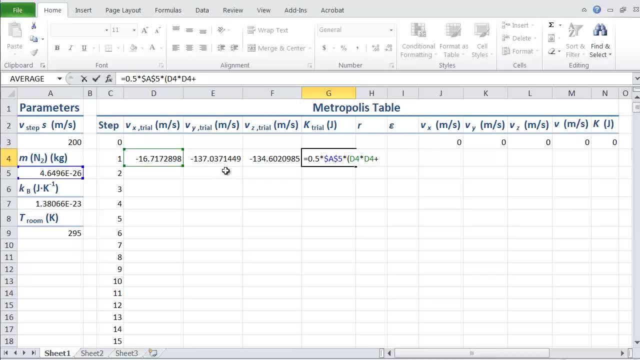 times vx plus vy, squared plus vz, squared close parens. okay, then we need the random number, which is just equal to rand, and we're going to use the same random number for all three components, so they're all being decided the same way. and epsilon, here is our boltzmann factor, which is: 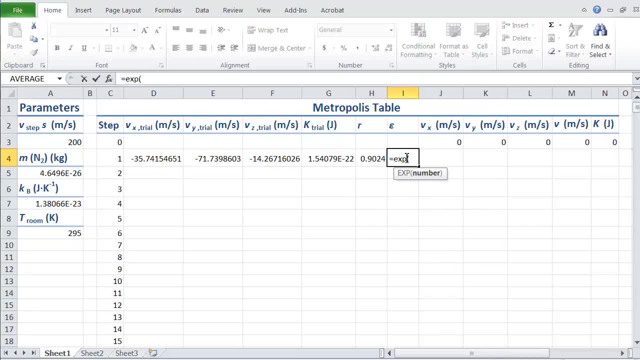 just equal to the exponential function times minus, and then open parens: the new kinetic energy minus the old kinetic energy, and then that divided by the quantity kb. oh, kb. hit f4 times t. hit f4 to get an absolute address. close parens, close parens. 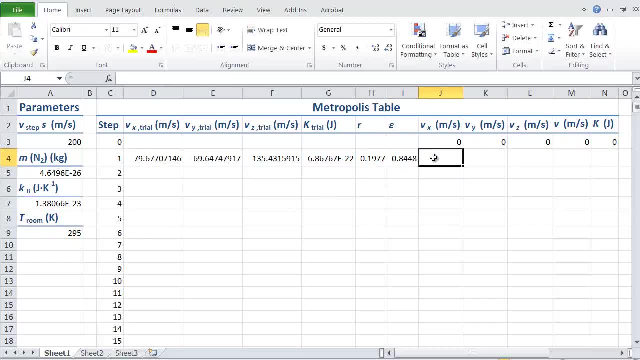 so that's our boltzmann factor. and then here what we need to do is use our metropolis criteria to decide whether we going to accept the move. so our new value of vx is going to be equal to, and then a conditional if- and the conditional is if r is less than or equal to epsilon, then we accept the move and use the new. 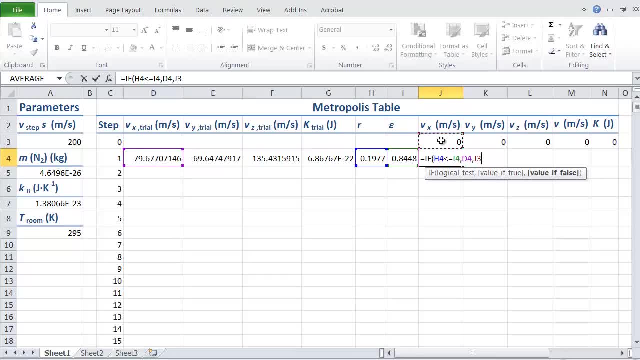 v, otherwise we use the old v close paren, and i need to do a similar thing for y, so i'll do that again. equals if and it's r is less than or equal to epsilon. if it's true, then we accept the old, the new value of y, otherwise we take the old value of vy. and then our last one is that: equals if. 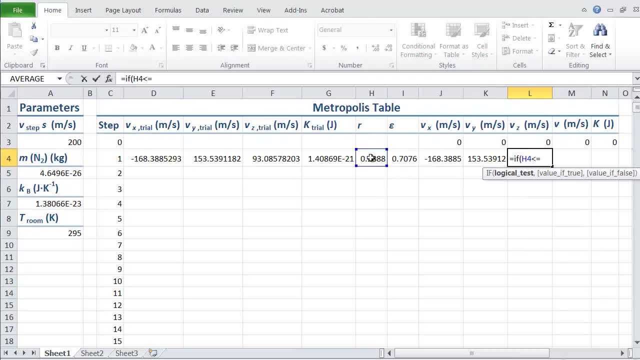 and again it's r is less than or equal to epsilon comma. take the new value, otherwise take the old value. all right, and these last two formulas should still work. so let's just copy those down. there we go, okay. so now we've actually filled in our first step. all the other steps are going to be exactly the same. so if I 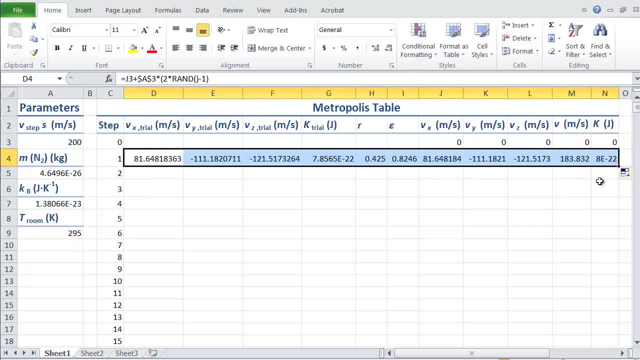 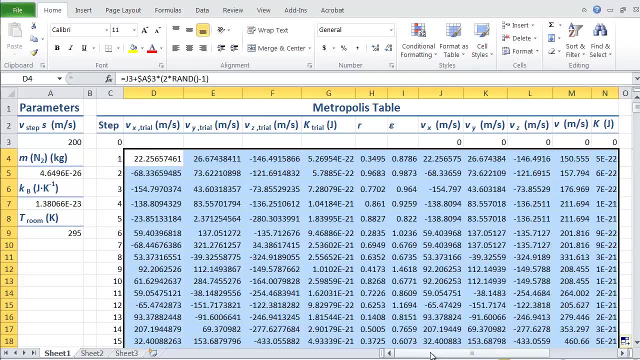 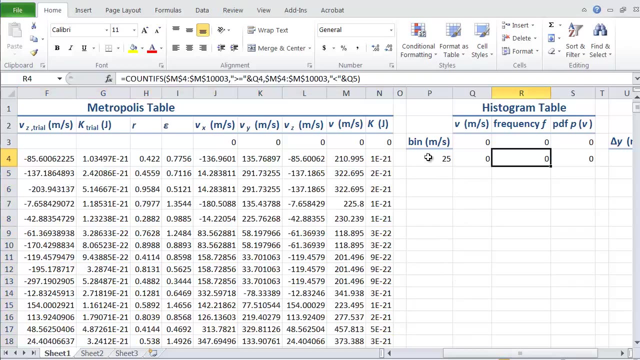 left-click, drag across the whole row and then get my open cross, change it to a closed cross and double click. I can fill in the whole simulation and if we've done everything correctly, it should be working all right. so let's now see if we can generate our histogram. so here's our histogram table. we have our bin, which is: 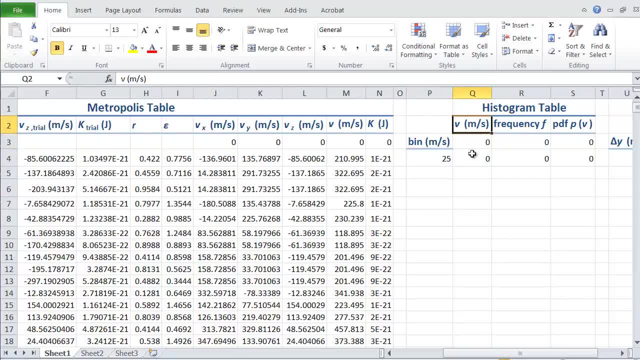 25 meters per second, the thing that we're actually going to be finding bins of which is going to be the the speed in meters per second. then we've got the frequency and then the probability density function, which is a probability density function of V. the first row has just 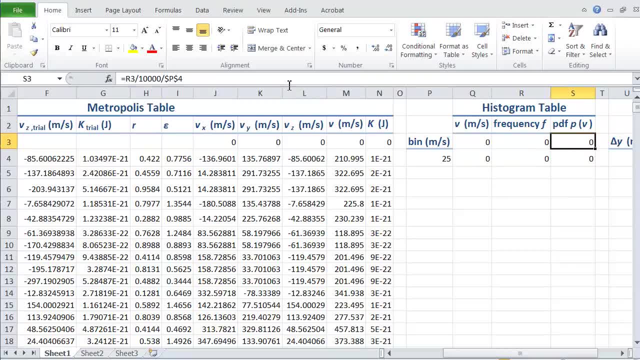 zeros in it. the probability density function, just to let you know, is being calculated from the frequency. we're dividing by 10,000, because we've got 10,000 values of V, and we're dividing by the bin size to give us a properly normalized probability density function. okay, so this one's pretty easy, it's just. 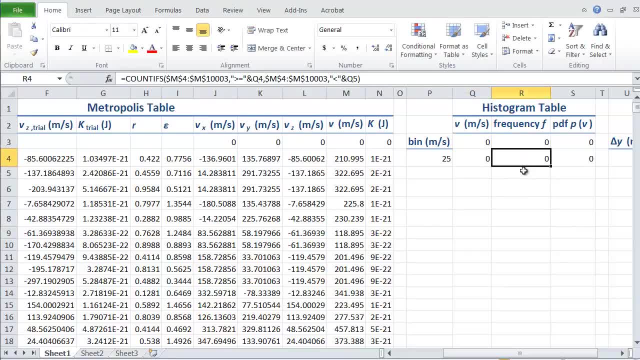 the previous value and the hardest thing here is the frequency doing the count. so this is based on the previous video and the one before that. let's just quickly go over what we've got. let's count ifs the range that we're looking at goes from step one for V all the way down to step 10,000. 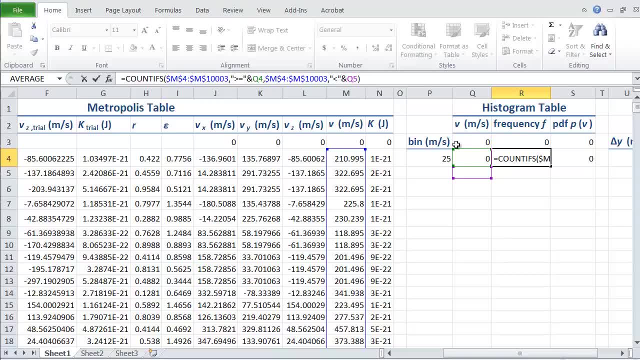 we're saying: if the value is greater than or equal to the green box, then count it, but it also has to be less than the one in purple, which is the one underneath. okay, so we're going to need that. so let's say what that is. that's going to be equal to the one above plus 25, and that has to be F4. and 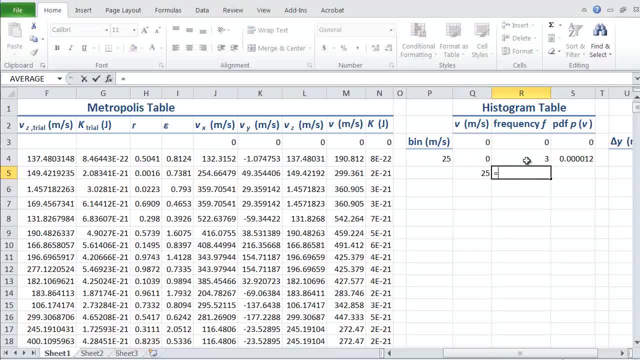 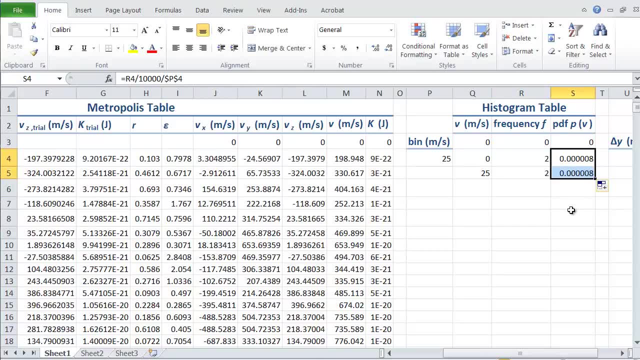 our frequency for this guy is going to be equal to the one above, and our value for the probability density will be the same. okay, so I can now copy down all of these and go as far as I need. I think I'm going to go out to about 1,500 meters. 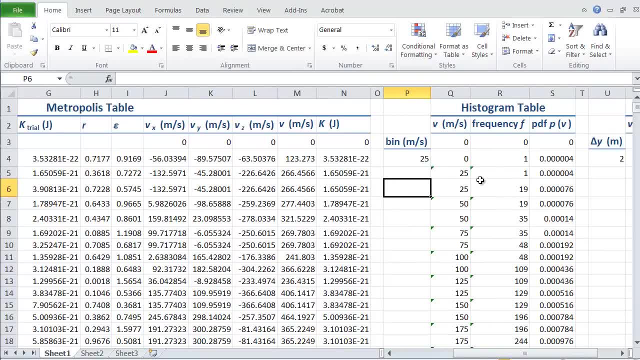 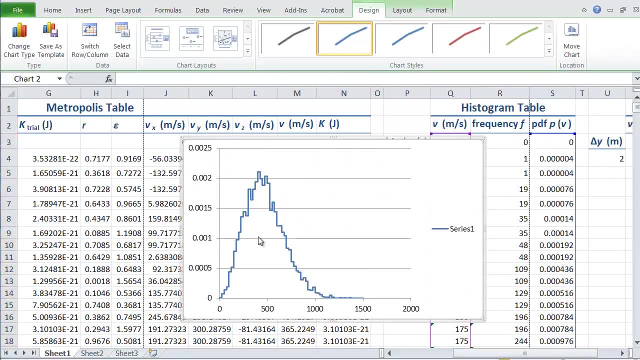 per second. okay, so let's see how we're doing. we've got speed and we want to plot it against probability, density, we need to insert and we're going to unskirt a scatter with lines. there it goes, and we want to format this, so I'm 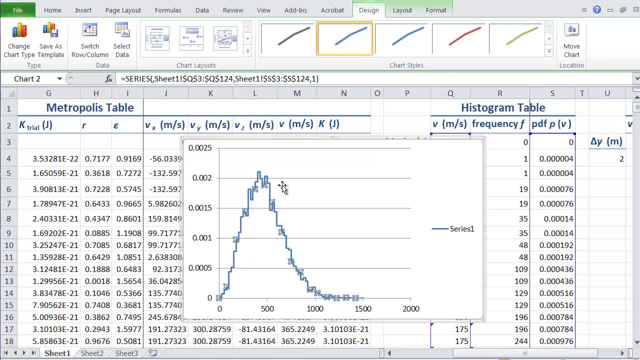 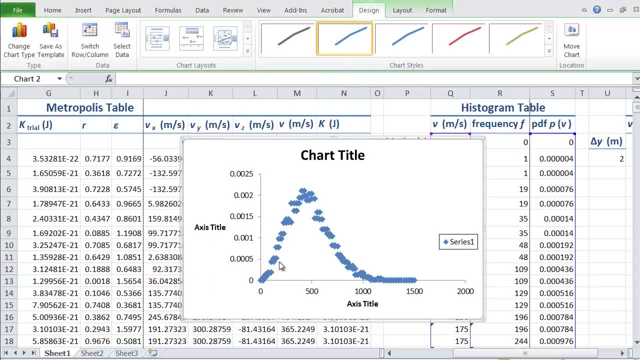 going to use my. what am I going to do? I'm going to use change chart type and use my template, and the one I have is markers only, which isn't quite what we want, so I'm going to go back and change it to be lines. okay, so now we have our probability density function, what I want. 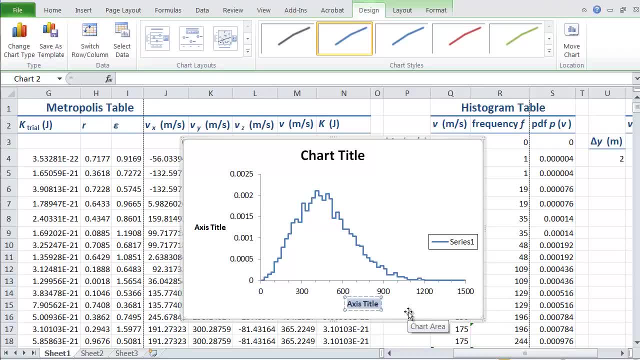 to do now is just tidy up the axes and give it a proper label- molecular speed and meters per second- and then I need to change the vertical axis to say what that is- probability, density- and you'll notice that the units are actually seconds per meter, so that this thing multiplied by that thing gives you 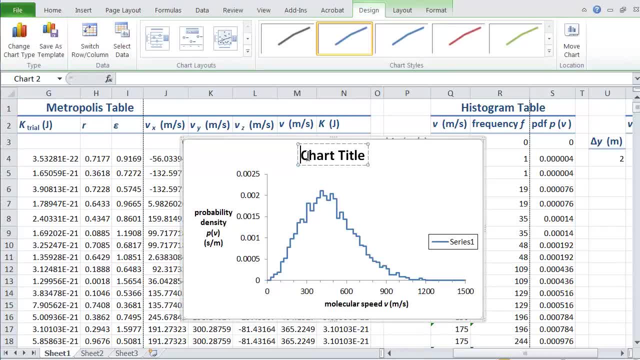 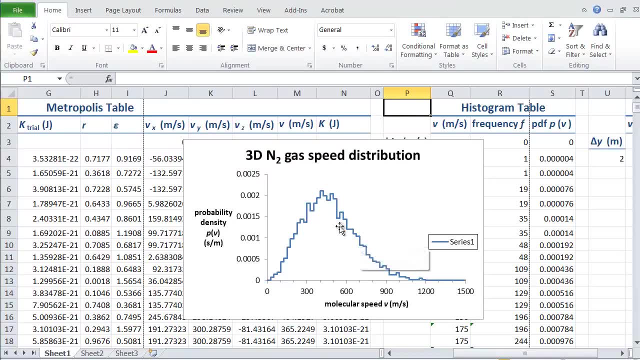 something without units, and then we need a decent title for the chart, okay, so now that we've got that entered correctly, let's just hit delete a little bit and see what we get. so we'll see that we've got a graph here that changes. so now that we have got some numbers, so we do need to do that too.